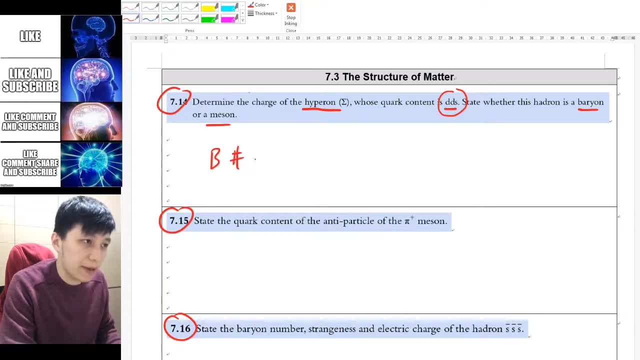 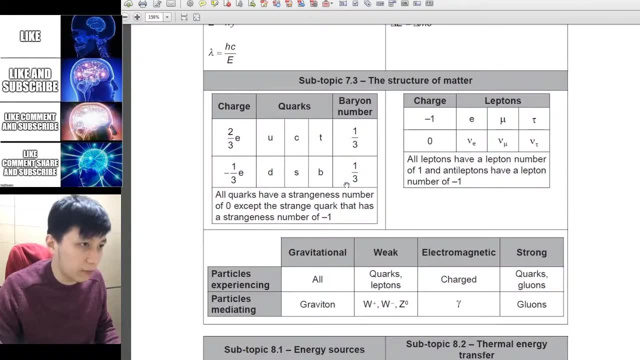 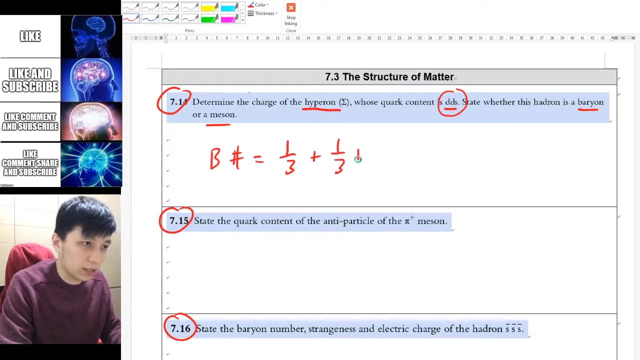 determine. this is all depending on the barrier number of this hyperon. So go and check it out. For D it will have a barrier number of, or actually all these are regular quarks. So if you remember or if you just check the data, 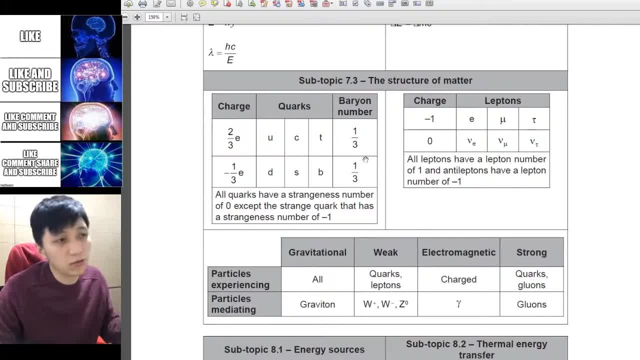 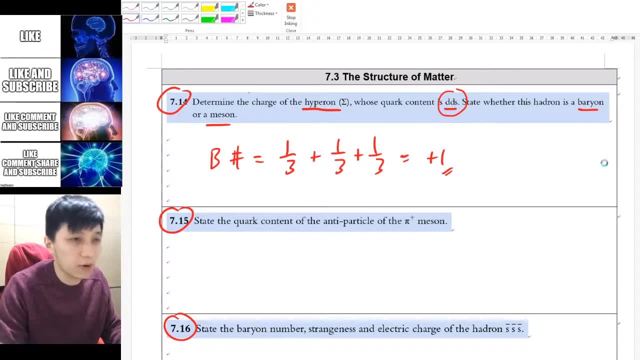 table all these, all six of these would just give you a positive number, 1 over 3 barrier number, And so that will give you a total positive 1.. So that's why the answer would be the baryon, the regular baryon, For meson the barrier. 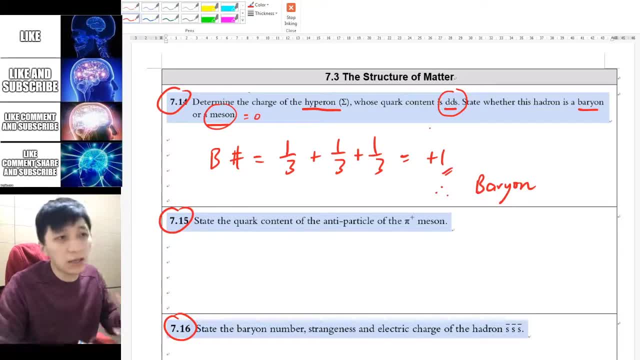 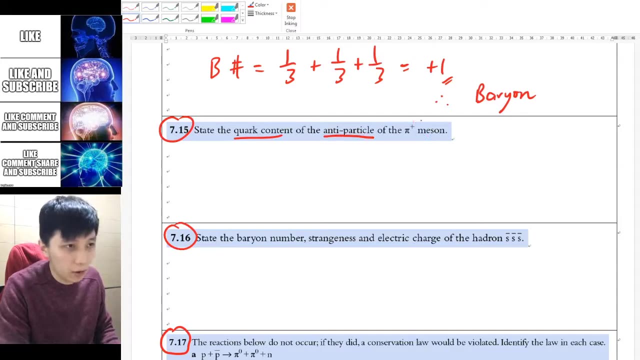 number has to be equal to 0. And obviously by looking at its structure you can already tell, because it should be something that has a regular quark together with an anti-quark. Next example: it asks you to find the quark content of the antiparticle of this meson. Let's talk. 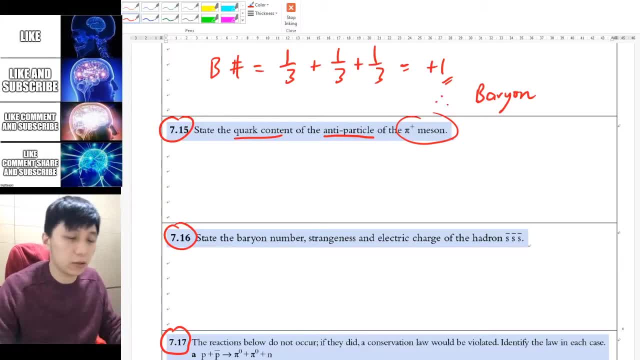 about January, how to find an antiparticle of a certain particle. So let's say, if you go back and revisit the quark content of proton, that will be UUD. Okay, so UUD is a proton And if you want to find the antimatter of proton, then it's. 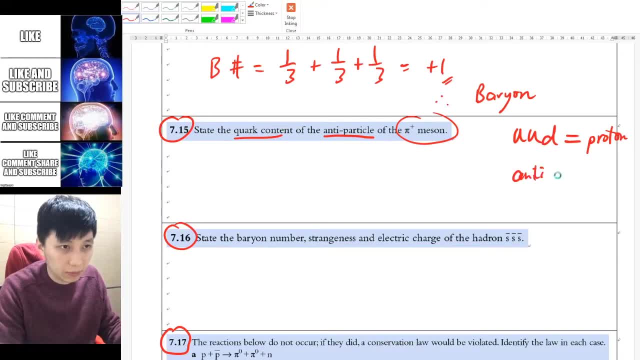 going to be simply getting each of these quantum to be its anti-quark. So NTU, NTU and NTD, and that is the simple trick, how you can make a particle: by finding its anti-particle, quark content of a certain particle. However, since you are not told the quark content of these pi positive, then you need to find out what is the quark content of these pi positive. Since then you need to go back and revisit the quark content of the anti-quark content, and you need to look at it carefully, And then you will find that you can go back and revisit the. 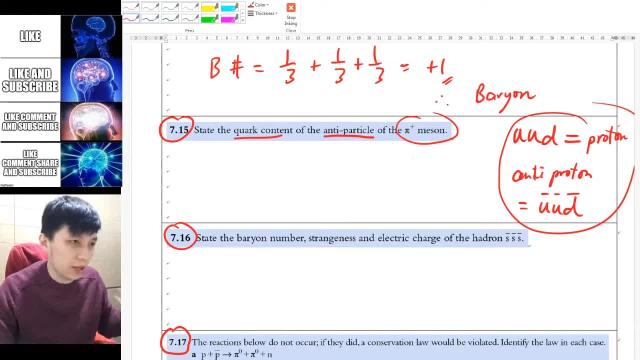 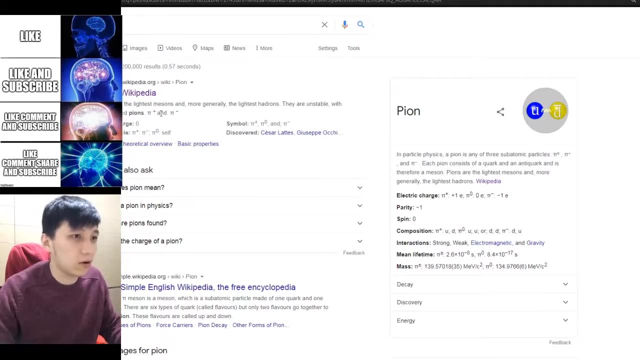 which is called pion officially, then there isn't a way that you can work it out. so this is the textbook spot. all right, this is from textbook. so this is the default form textbook. they should give you the correct content. so in this case, let's just go and google it. so this is called pion p-i-o-n. and if you go, 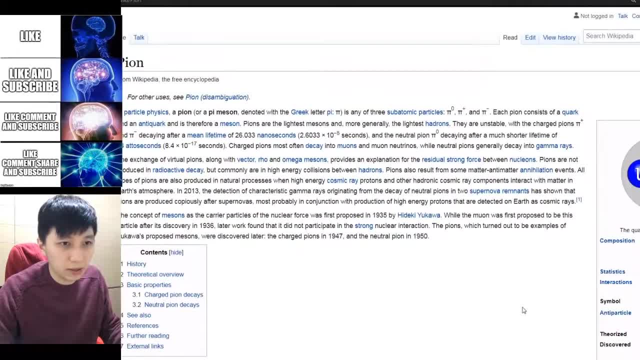 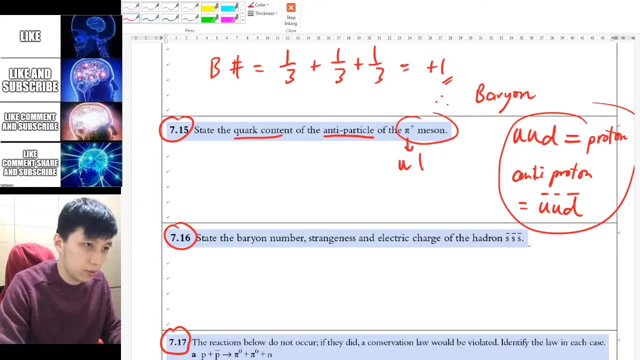 into it and you will find on Wikipedia that it's going to be UNTD. so let's put it down: this is going to be UNTD, and so for its NT pion. all right, let's just write it this way then the content is simply we kind of. 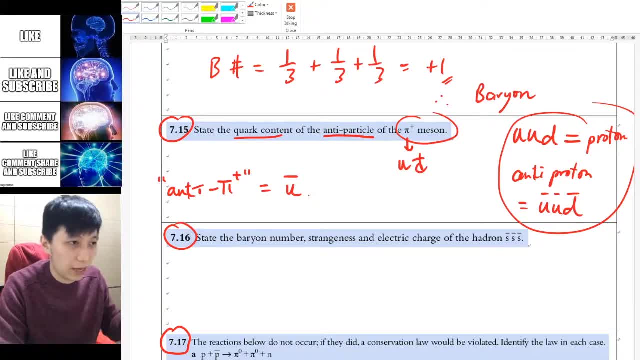 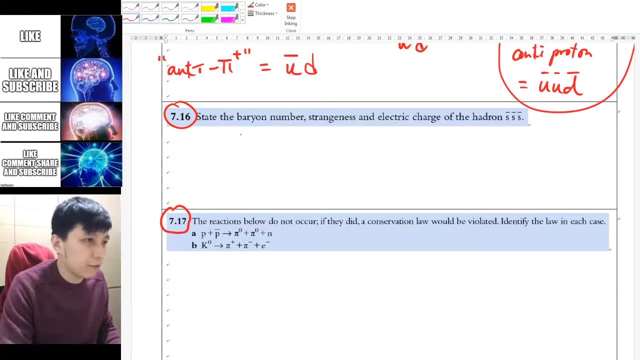 reverse the quark so this will become NT up and this will become the regular down quark next up. we ask you to find a better numbers strangeness, which is something that we haven't mentioned, but i think if you are smart enough you'll be able to find it from the data table and just apply it simply, and the charge number as well. 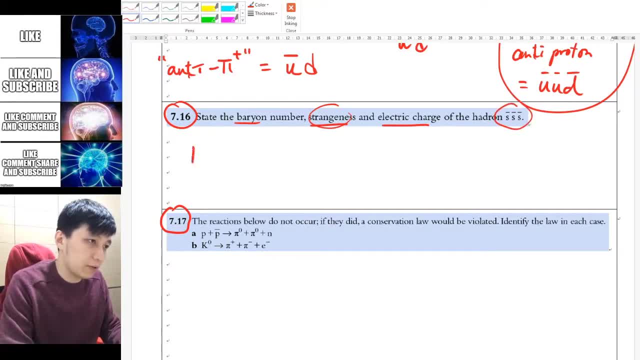 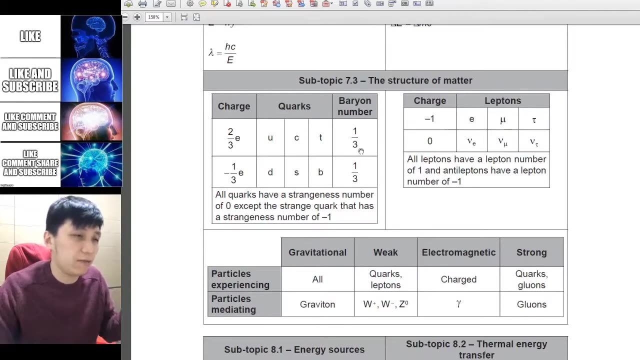 for this hedron, so obviously for the barrier number. allow me to write in this notation, but don't write in exam. these are all anti-quarks, so if you like to or if you don't remember, you can go back and check out. these are regular quarks and they carry positive one over three. they run. 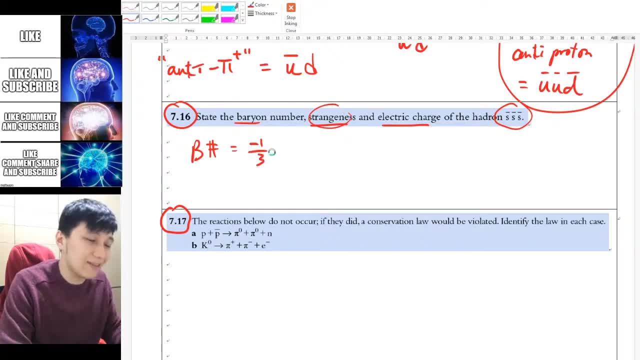 them, and so for these, these, each of these will carry negative one over three, because these are anti-quark and so you're like having all these three act together, and so this will give negative one. so obviously, this is a, this is an anti-barrier. as for charge number, let's do it first, which is something that you should know. 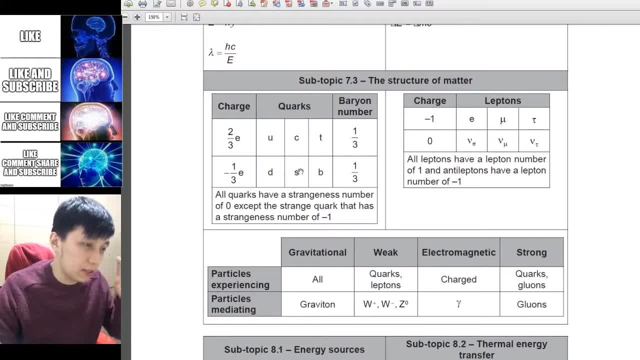 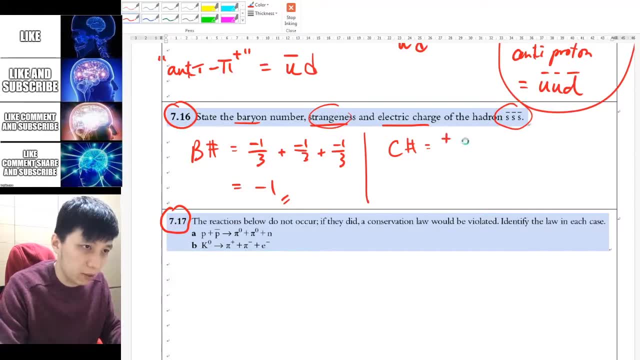 go back and check out the data table and you can see the regular strange quark is going to be negative one over three, and so for this one it's going to be positive one over three, and then you just add them together. you can just multiply by three, but i like to write this way, which is clear: 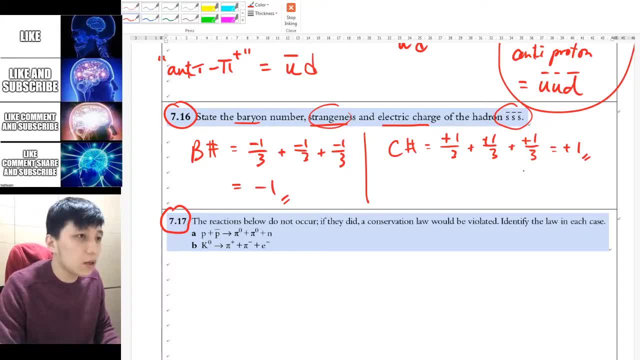 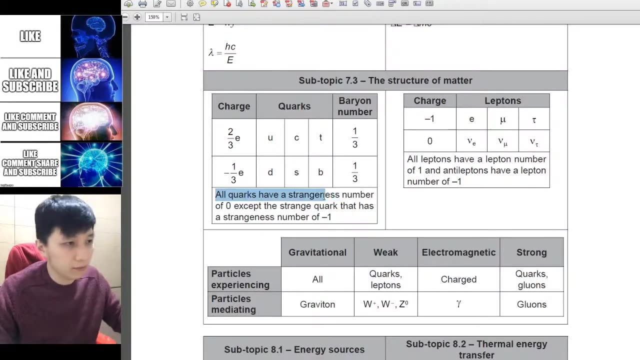 to see. so charge number is positive one. lastly, strangeness, so something that you need to read from the data booklet simply and you don't have to memorize it. so according to the sentence here, all quarks will have strangeness number of zero. that means you just ignore it. so for all these six quarks you 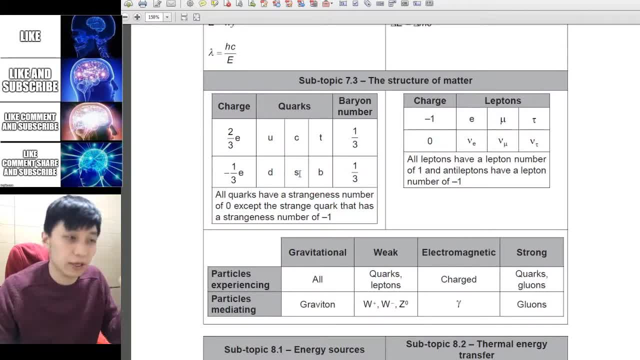 only have to care about strange quark for its strangeness, obviously. so nothing that is complicated. so for a regular strange quark it will have a strangeness number of negative one. okay, so this is what it said. this is the game rule. sorry, please don't ask me why it's not positive one, because i don't know. all right, if anyone know. 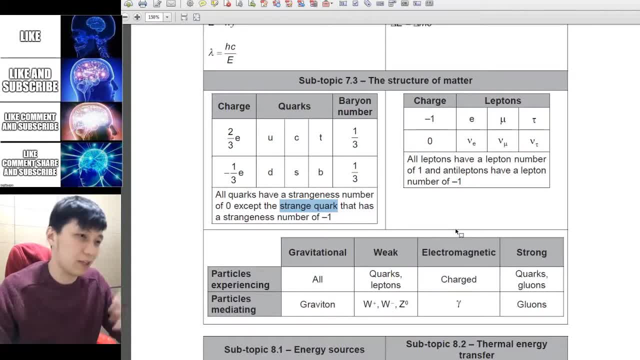 let me know in the comment section below, like why it is not defined as positive one, but not but negative one here. is that anyway? so, since for regular strange quark it's going to be negative one, but then we've got anti-strange quark right, so it's going to be an opposite, the reverse of. 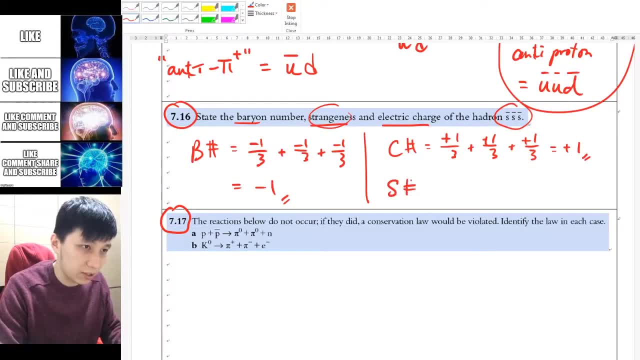 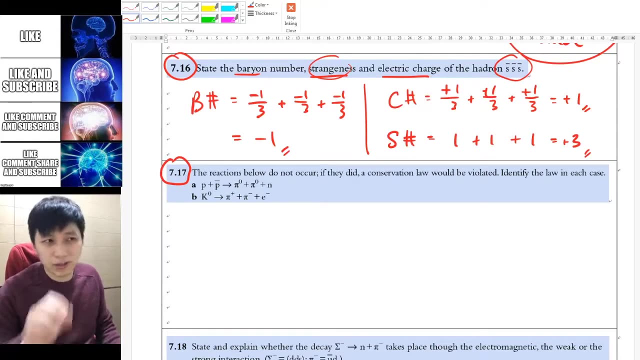 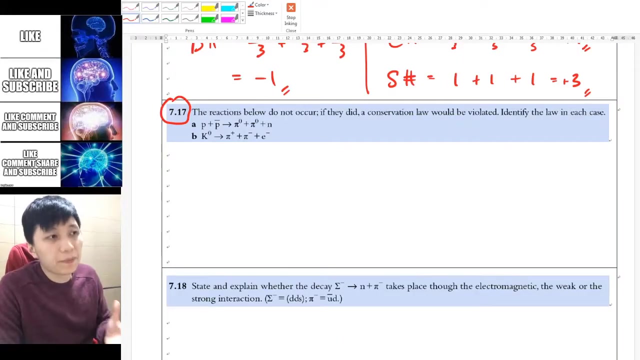 negative one. so that means for strangeness we will have positive one, positive one and positive one. that means three positive in total for strangeness. we'll talk more about it in the next video later on. they don't always concept and that's why it is very strange. 17 is a very typical question that you may see in the 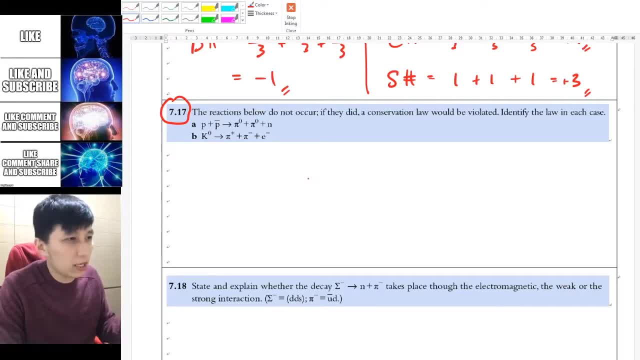 ib physics exam. they provide you a reaction and ask you to check whether or not it is possible, and you can check it by using the conservation law. so the conservation law that you need to check will include burial number, charge number or which are the two that you have learned, obviously, how to. 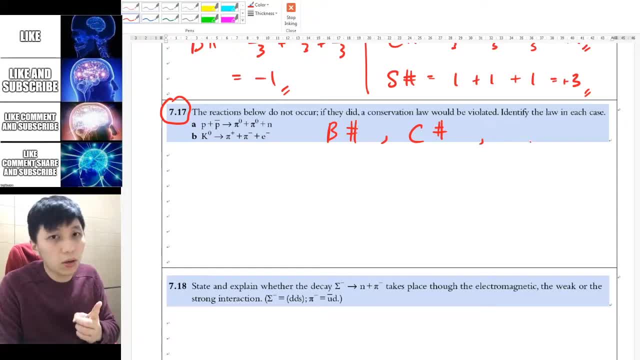 read from the data table. and there's one more, guess what? not the strangeness. okay, like what i said earlier, they don't always conserve, and that is some other trick, some other rule that you have to look um to check it out. the other conservation law that you have to check is called laptop number. okay, and that is. 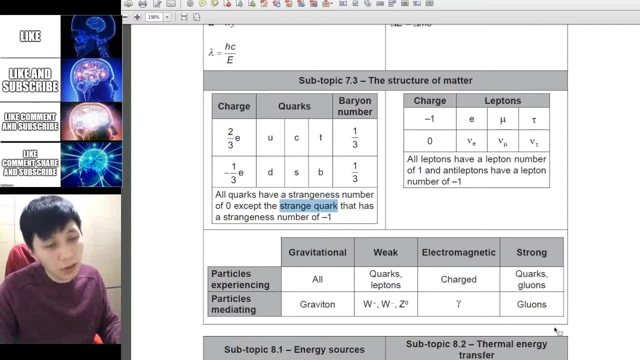 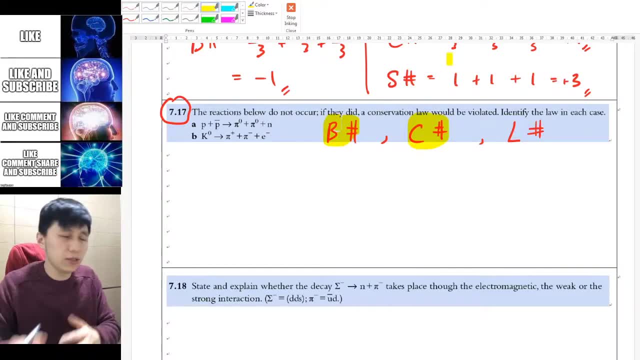 something you can find from the data booklet also. but then in this question i think we will only need to focus on the first two, okay, so let's just focus on the first two for this question first. okay, so for easy representation i'll split this space into two and i will do part a here and 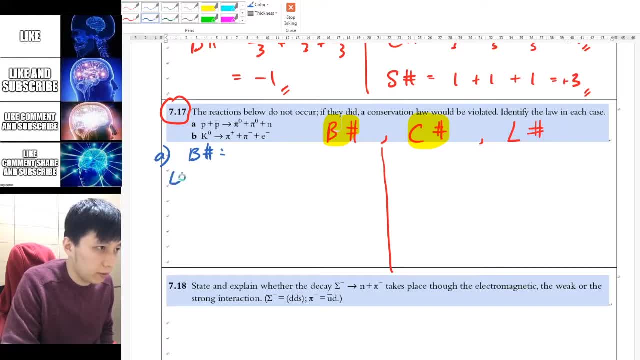 let's do barrier number first. okay, so for left hand side, the barrier number is going to be proton and anti-proton. so, as you know, proton and a proton, they should each have one and negative one, or even if you don't know any symbol in any of them, it's all, it's going to be cancelled out. 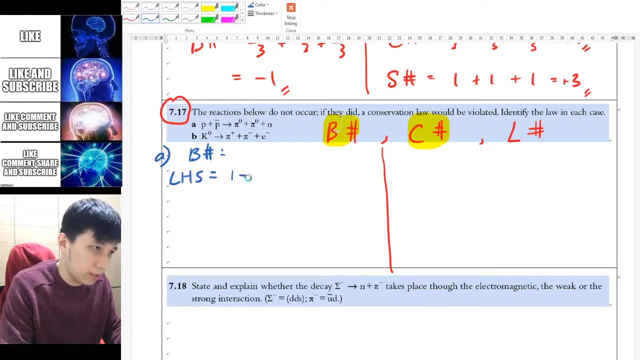 anyway, right, and so that must be zero at the end. so for me i'll put down one plus negative one that will cost you zero on right hand side. let's check. so again, these are pion, and if you recall how we check out on wikipedia, then you may recall that they are mason if you look at. 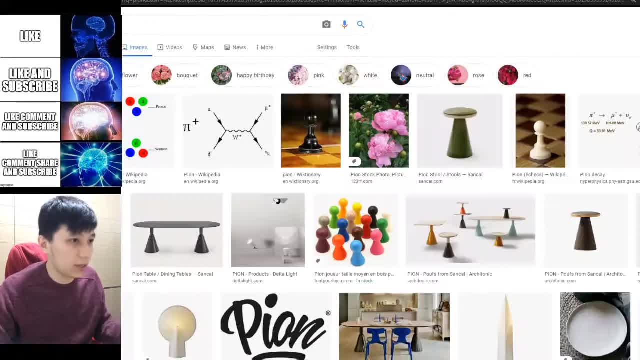 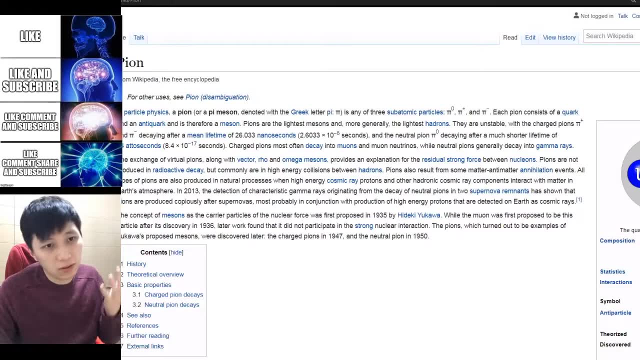 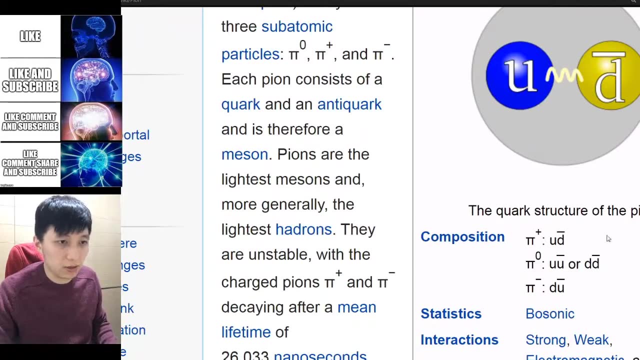 their structure. you know they are made of a quark and anti-quark and so obviously no matter it is positive, neutral or negative, because they could be at a different form, as you can see here, right, but then no matter what they are, they are just a. 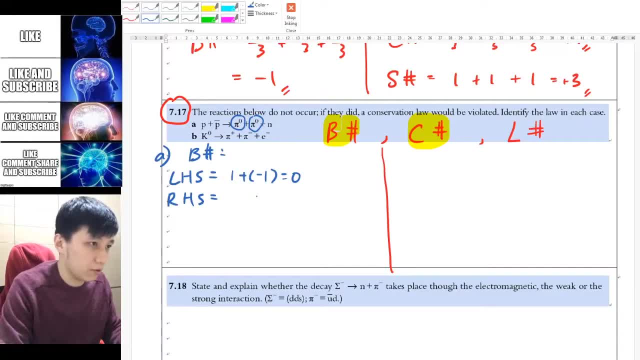 mason at the end of the day. so for barrier number is going to be zero plus zero. and lastly, this one is an n referred to neutron, so it's going to be positive one. so at the end you have one. so that means, uh, left hand side does not equal to right hand side and therefore, um, the barrier number. 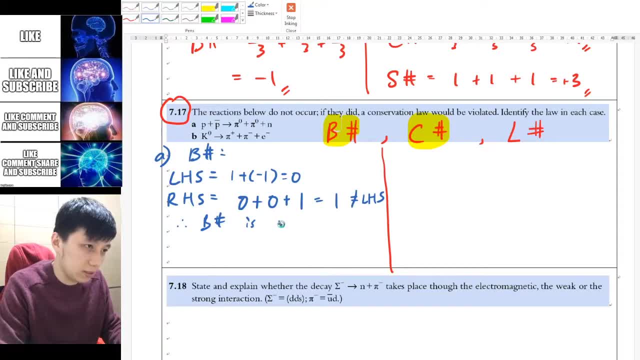 or barrier conservation law is violated. similarly, we can check the charge number. and so for left hand side, we have again proton, antiproton. so again you know, proton will be positive one and antiproton is going to be opposite, so negative one. so again it will be zero. for right hand side, we can see this is neutral. 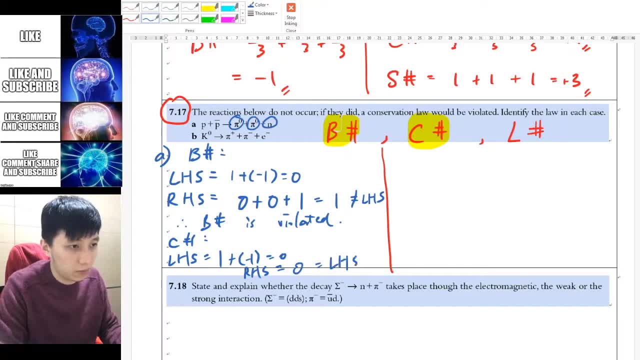 neutral. so yeah, obviously zero. so okay, this part is fine for charge number all right. part b: let's do again, barrier number first, and so we will have left hand side having a symbol of k zero. so in case you don't know what it is- and again, it is default by the question that they should have- 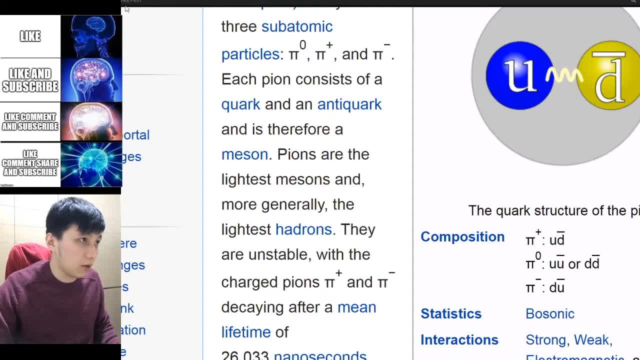 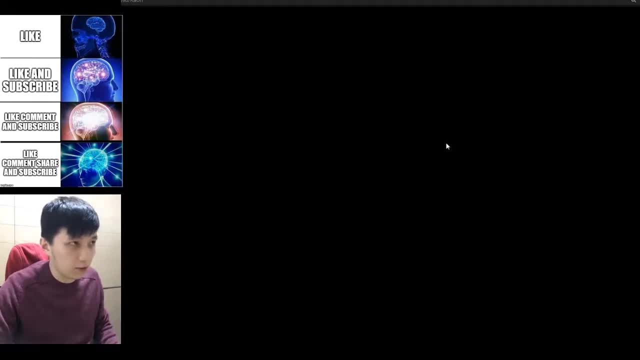 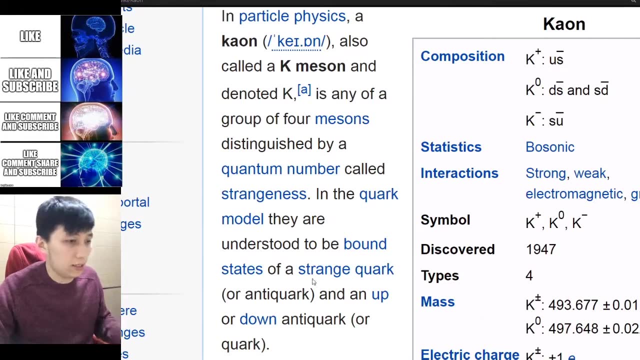 provided you the quark content. and so, uh, what we can do is i can tell you that this is called cai on, and you can find the quark content on wikipedia also is again, you can see, it's a kind of mason, you nts, and so obviously for besser number is going to be. 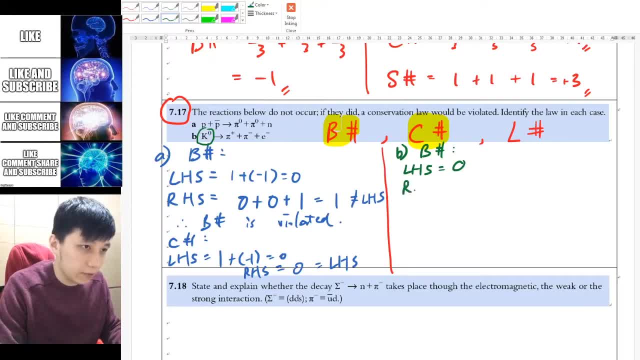 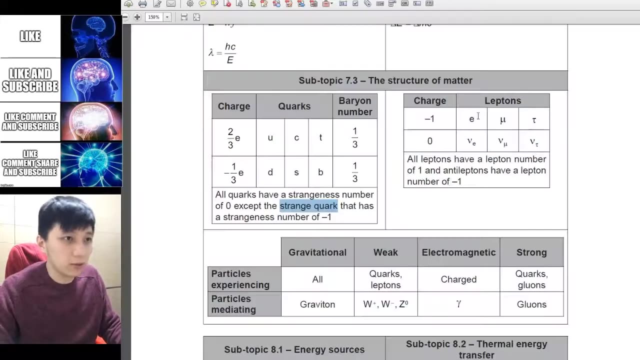 zero, because this is a maison. and then from right hand side, uh, again, these are piles, so pion will be zero. and then you can see, here is an electron, and if you recall what we have talked about earlier, that electron is a kind of laptop, it doesn't. 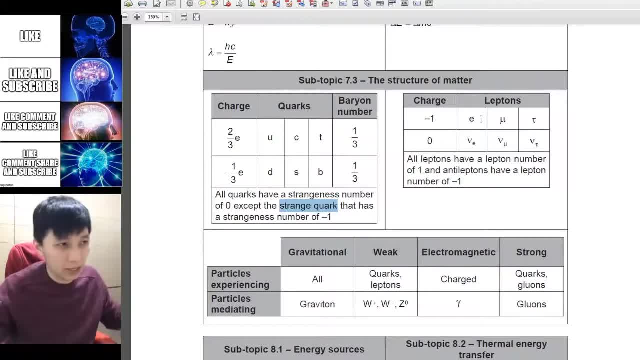 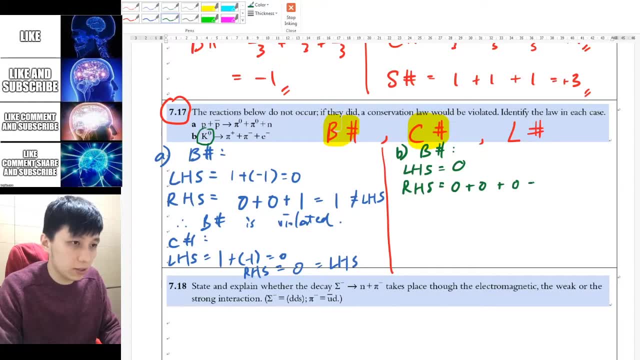 even belong to Hedron or contain any quarks, and so for barrier number, obviously it is also zero, okay, and so that would equal to left hand side. so for barrier number, the test is passed. now let's go for. the charge number for left hand side is going to be neutral. as you can see, is k0, so 0 actually means 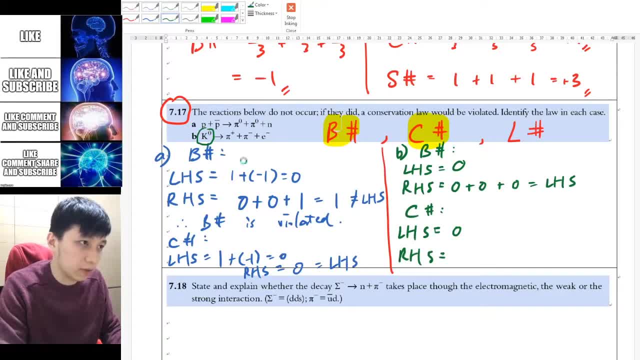 neutral here and right hand side, we have got positive 1 and then negative 1 for these two pion and then for electron is of course negative 1 also. so eventually you have negative 1, which does not equal to left hand side, and again you can say: 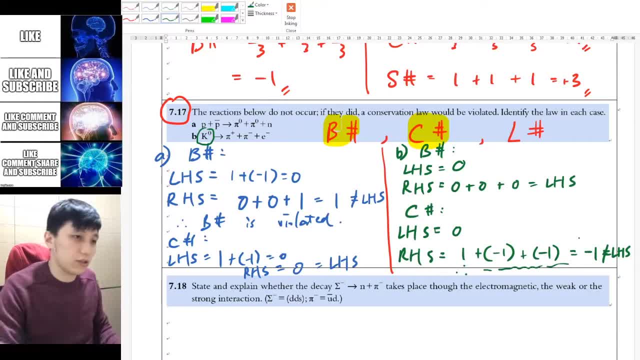 the conservation of charge is violated. and last but not least, all right, actually I think this is good enough. if you have finished all these things, we have laptop number, and that's something we again haven't mentioned and we'll probably talk about this in another video, two videos later on. but then for B, it actually has violated the. 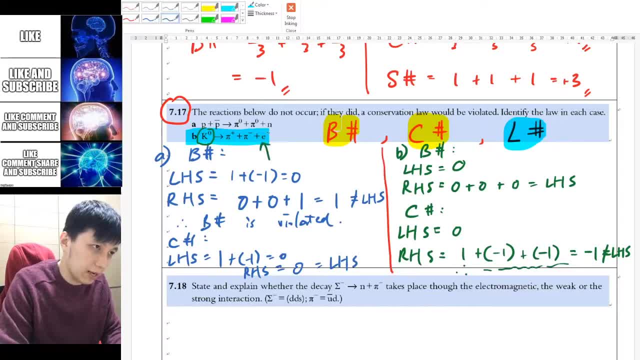 laptop number because that's something to do with the laptop, the only laptop you can find which is the electron. here on the left hand side you don't see any laptop all right, and on the right hand side this is the only one that also. obviously, this is also violated. so if 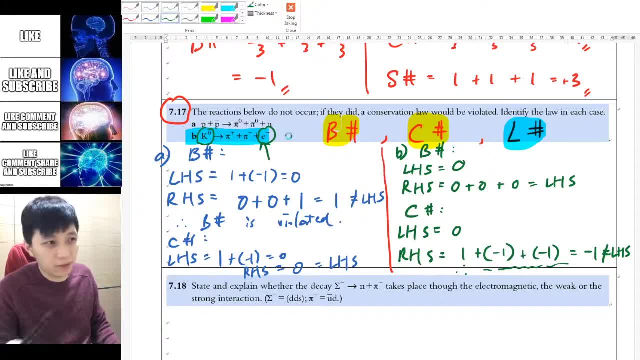 you have find that, then yeah, you should be happy. and that's something extra. yeah, fine now.